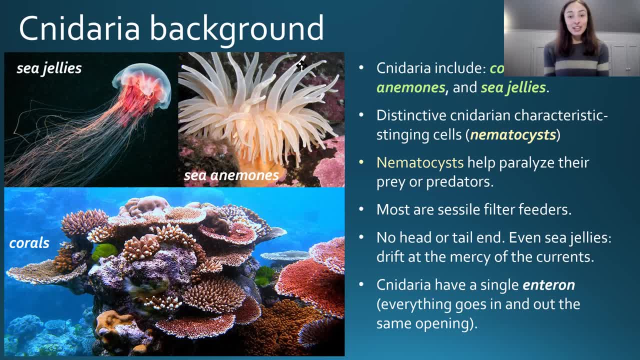 focused on in a paleontology class or, for example, in this video, is because in paleontology, which is the study of ancient things that become fossilized, we have to focus on the things that actually can fossilize. Sea jellies and sea anemones don't have hard skeletons and therefore 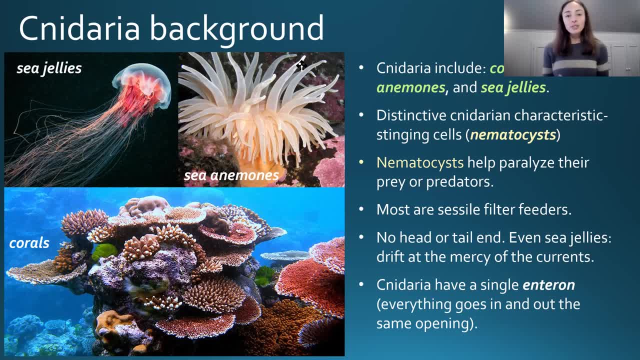 don't get preserved very often in the fossil record, And so corals have a very extensive fossil record, and for that reason we'll be focusing mostly on them in terms of classification, fossil record, morphology, etc. in this video. However, we will touch on all three groups as we discuss. 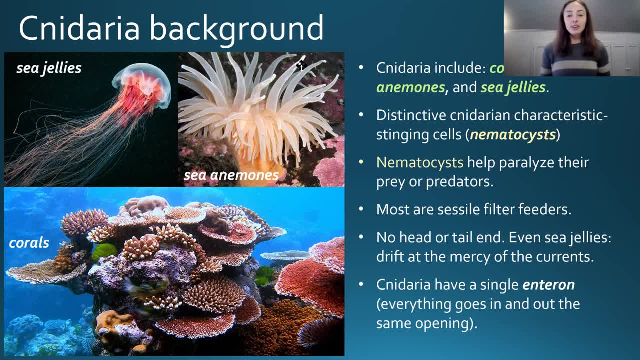 how Cnidaria reproduce and their ecology, etc. before we get to the paleontological details. So, in terms of Cnidarian distinctive characteristics, one common characteristic that all Cnidaria have is nematocytes, or stinging cells. These stinging cells help to paralyze 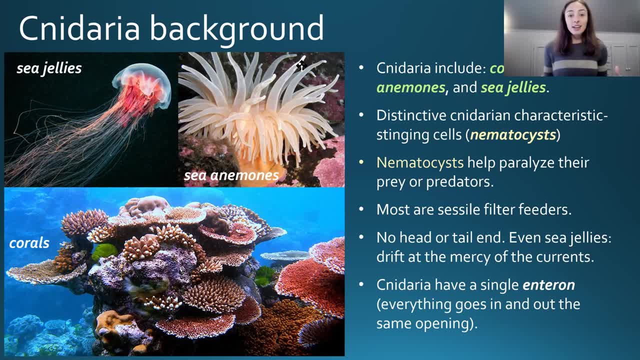 their prey or predators, and this is a beneficial characteristic that helps them live longer and reproduce more, and therefore more evolutionarily successful. Additionally, they are mostly sessile filter feeders and they have no head or tail end. This is even true for sea jellies. 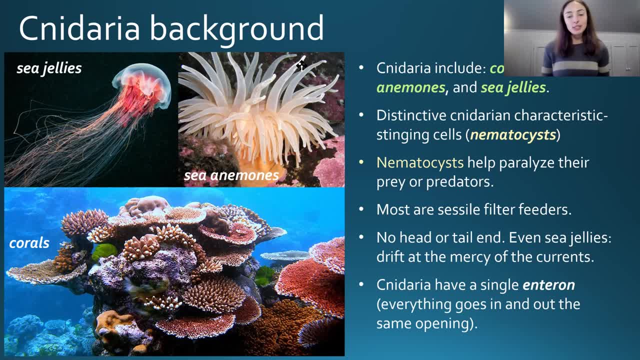 or, as you might know them, jellyfish, but the more technical term is sea jellies, which may not seem technical, but they're not fish. so they're sea jellies, Even these animals which seem to be going in one direction or the other when they float. 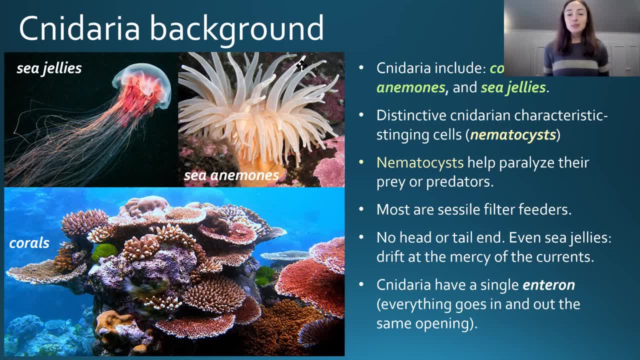 they are actually just drifting at the mercy of the currents. It doesn't matter to them which direction they're facing, because they have no head or tail side. Lastly, for the general characteristics of Cnidaria, they have a single enteron where everything 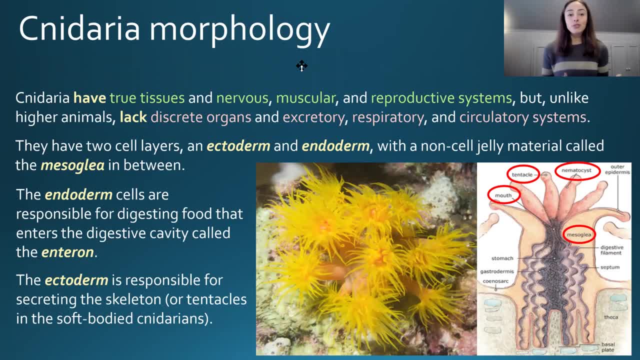 goes in and out the same opening. Now to get into their morphology. Cnidaria have true tissues, nervous, muscular and reproductive systems, but unlike higher animals they lack discrete organs and excretory, respiratory and circulatory systems, So they're a little bit more complex. 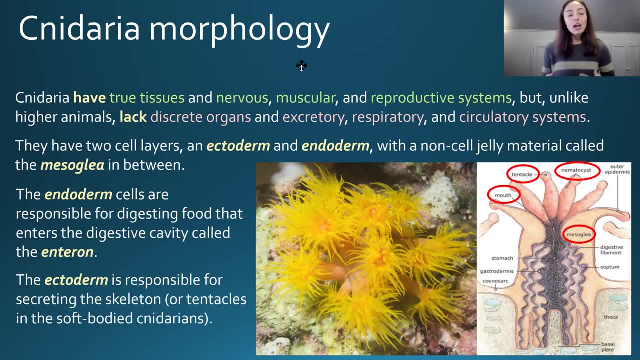 than the last phylum we went over, which is Periphera or Sponges, but they are not as complex as further phyla that we will go over later in the future in terms of invertebrate animals. Additionally, they have two cell layers, an ectoderm and an endoderm, And in between, 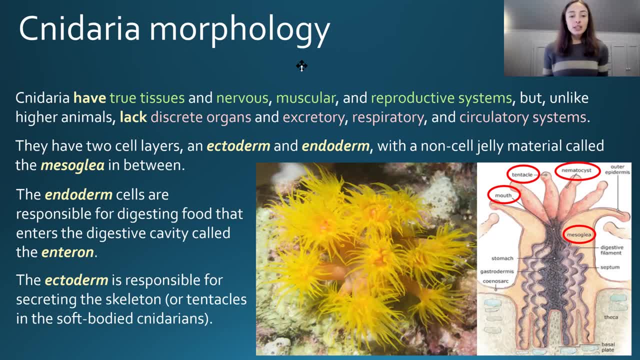 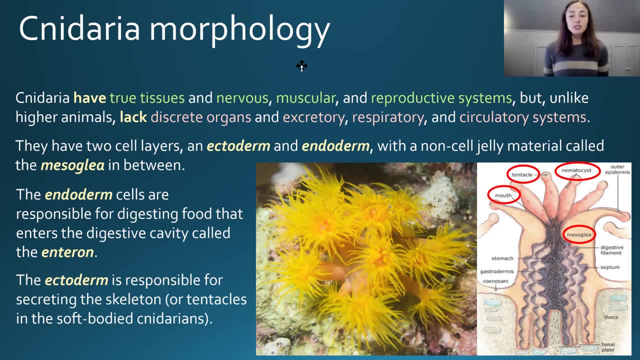 endoderm cells are responsible for digesting food that enters the digestive cavity, or enteron, like we talked about in the last slide, and the ectodermic cells are responsible for secreting the skeleton. in a Cnidaria that has a skeleton like corals, for example, But in the soft body. 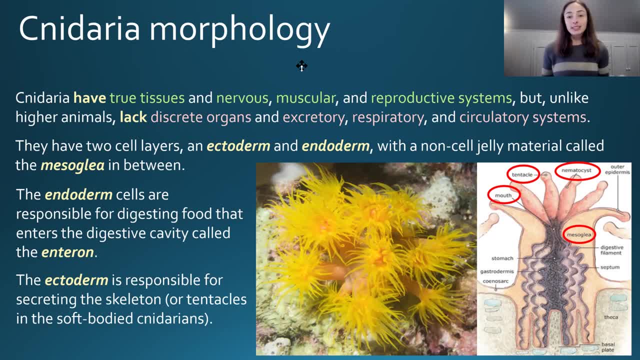 Cnidaria. the ectoderm is just the outer layer of skin and secretes things like tentacles instead. So if we look at the figure to the right here, we have some of these characteristics circled in this diagram. We have here the mouth or enteron, and then the stomach, and then we have the mesoglia in between the 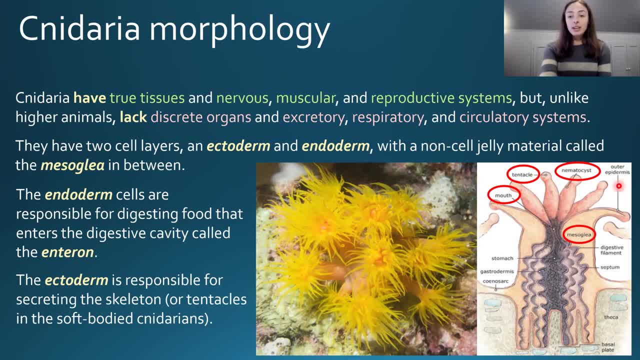 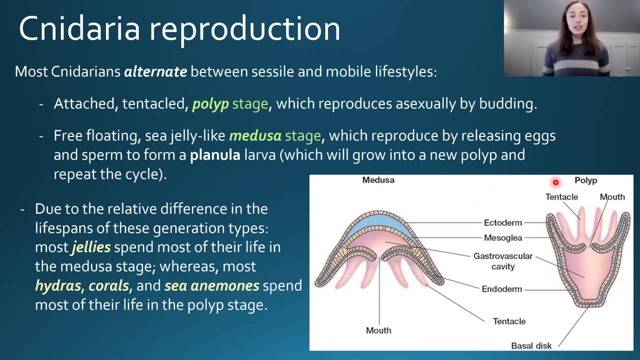 endoderm and the ectoderm, and then we have the ectoderm containing the nematocytes, which are the stinging cells, and these stinging cells coat the tentacles which are made up of the ectoderm. So now that we have a general idea of the morphology or body layout or anatomy of Cnidaria. 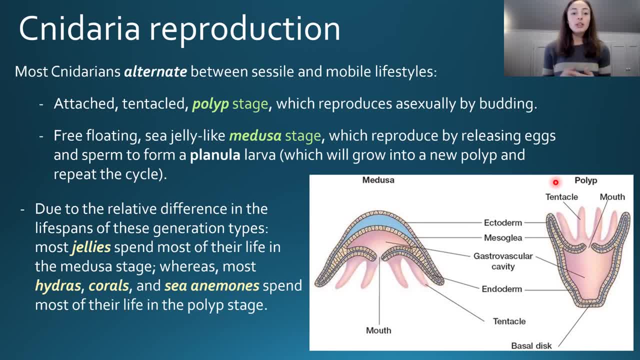 we can talk about reproduction a little bit. So in terms of Cnidarian reproduction, most Cnidaria cells are made up of the endoderm, and then we have the endoderm, and then we have the stem cell, and then we have the endogestin, and then we have theится cell. 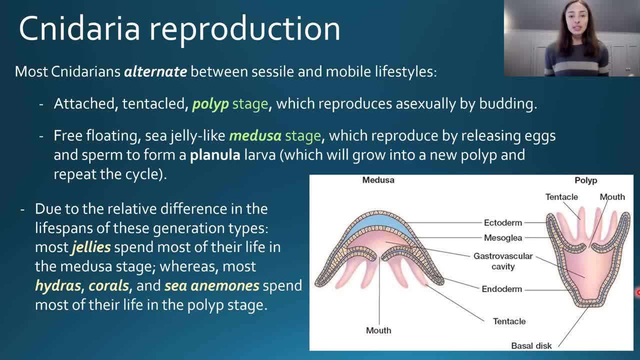 They all have different basic behaviors and so we want to be able to see the difference in how their life styles and ife circa wa word vit- Start with the low-piped menace, because we understand all of the different color variants. So we're all going to focus now, then we're going to focus on the의. 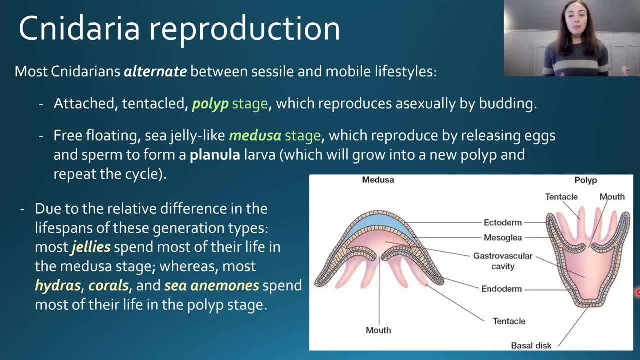 form, a planula larva, which can grow into a new polyp and repeat the cycle- and due to the relative differences in different types of cnidarians- most jellies spend most of their life in the medusa stage and most hydras, corals and sea anemones spend most of their life in the polyp stage- 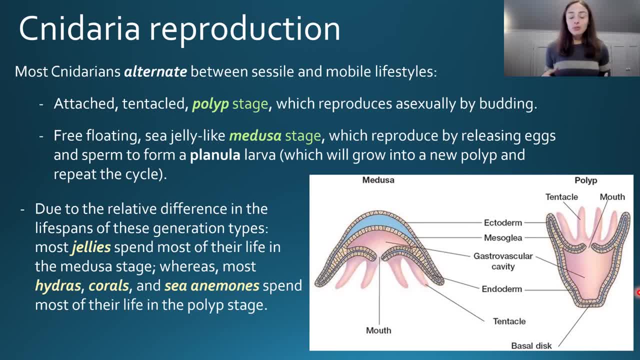 attached to a substrate and, in terms of distinctive morphologies of these stages, they might seem like they look very different if you think about a polyp jelly versus a mobile sea jelly. however, if we look at their actual structure, we can tell that if we just flip the polyp over and 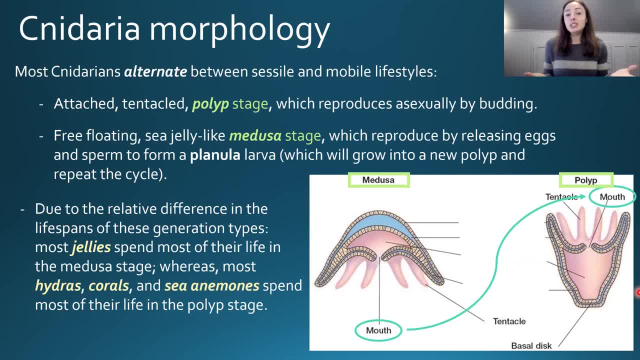 detach it from its surface, it looks quite like a medusa, and this is just to indicate how similar they actually are and to go over some of the other shared characteristics. in this figure we can see that they both have an ectoderm, a mesoclia, a digestive cavity, an endoderm and a mouth or enter. 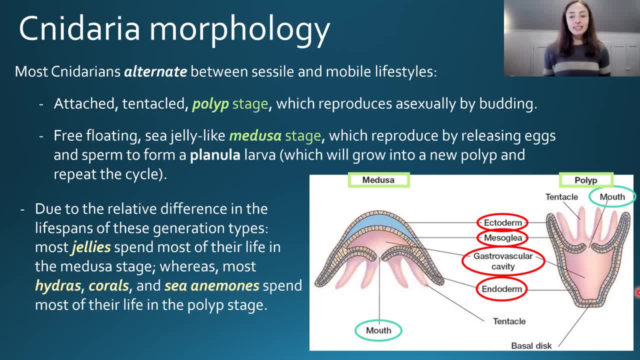 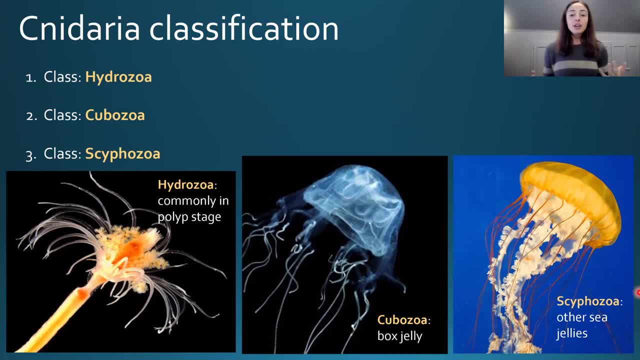 on, and so they're very similar, regardless of their stark differences in lifestyle. so getting into classification, just so we know what they look like, they're very similar regardless of their stark differences in lifestyle. so getting into classification, just so we know what they look like, we can understand the different main classes of nidaria. we have here the first three classes. 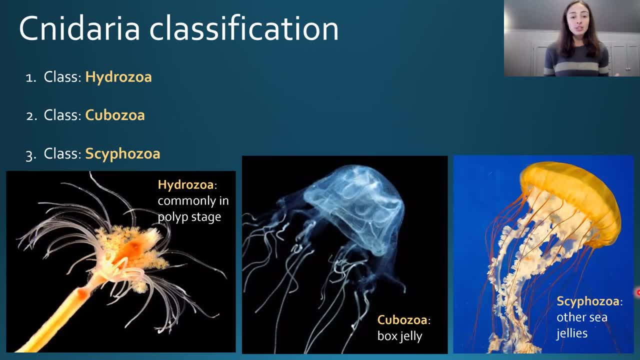 which are hydrazoa, which commonly remain in the polyp stage, cubazoa, which include common box jellies, and skyphozoa, which includes a lot of the other jellyfish or sea jelly species. but, as we can see on this page, these all look pretty soft-bodied. so what about the hard-bodied? more paleontology. 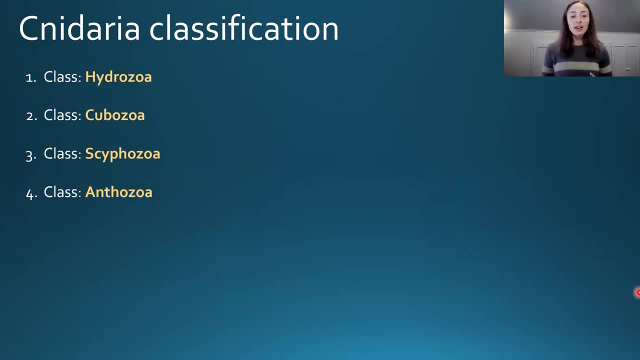 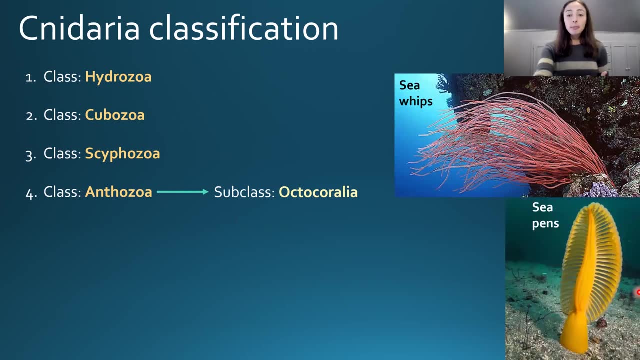 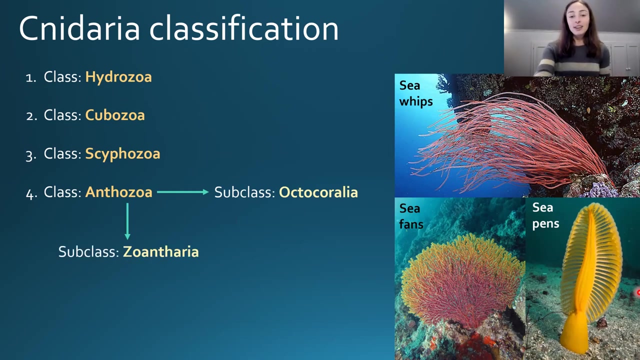 applicable nidaria. well, these are in a class called anthozoa. anthozoa includes a subclass, octocoralia, which includes things like sea whips, sea pens and sea fans, which have a pretty good fossil record, but the best fossil record is seen with the zuanthiaria. zuanthiaria include 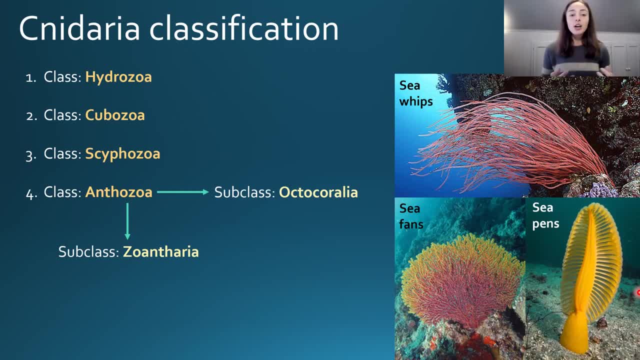 the three main types of corrals we'll be talking about, which are all orders. so we have phylum, nidaria, class anthozoa, subclass zoonzoa, and orders tabulata, rugosa and scleractinia. so to get into each of the 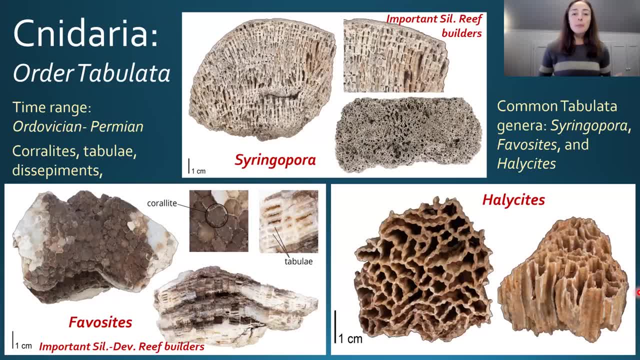 in more detail. we'll have a slide on each. So first we'll talk about tabulata. These were the first corals to begin to dominate in the early Paleozoic. They evolved in the Ordovician and they existed until the end of the Permian and went extinct during the Permian-Triassic extinction. 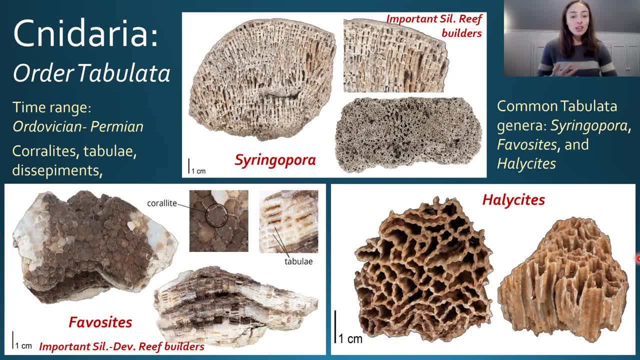 We can see in the structural picture to the bottom left that they have corallites, tabulae and decepaments, although decepaments are not labeled here. But basically the corallites represent each skeletal cup, if you will, from each of the polyps in the coral as a whole And 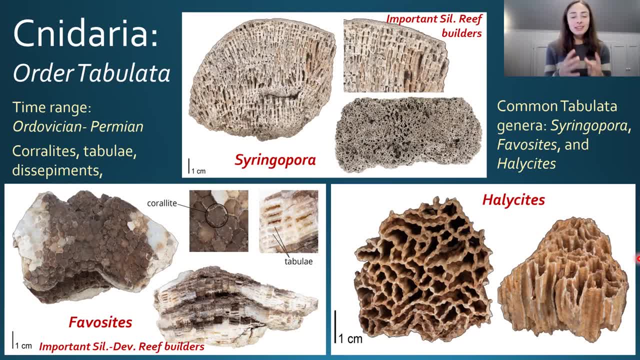 so each one of these little cups in the skeleton, or polygons in the skeleton, represent a preserved corallite structure. And then we have the tabulae, which are these horizontal table-like layers or laminae in each one of these tabulate corals, And this is why they're called tabulate corals. 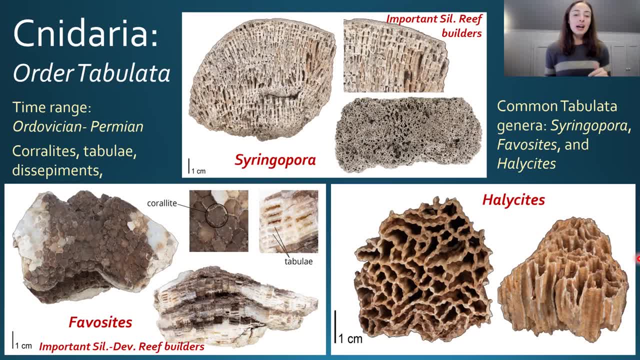 And then they also have decepaments in some tabulate corals where they have vertical separation In between their tabulate. The three main types of tabulate corals shown here are the genera, which is the plural for genus syringiomorpha- on the top, which looks like a bunch of straws. 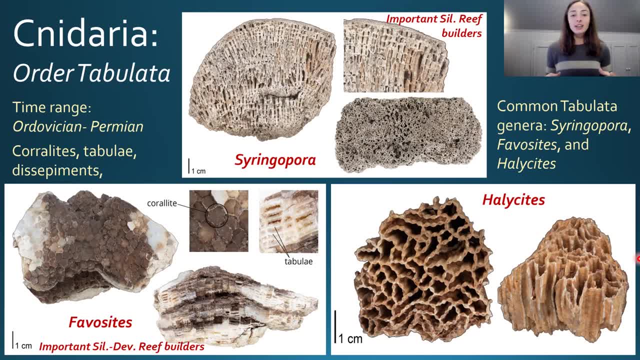 held together And these were important refielders in the Silurian. And then we have favicites on the bottom left, which is the one we were looking at, the structure, And these were important refielders in the Silurian to the Devonian. And then we have halicites to the bottom right, 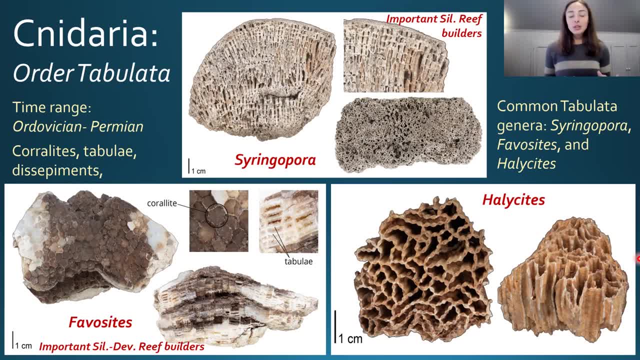 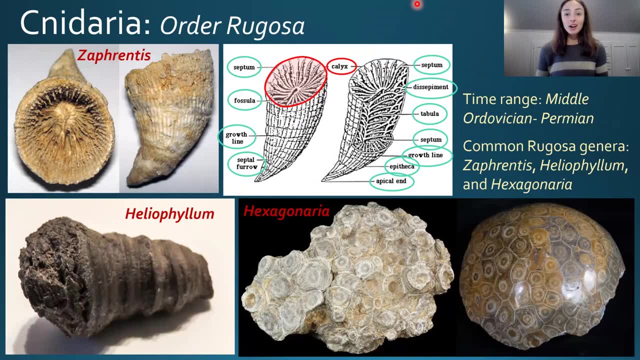 which were never dominant in reef building per se, but they were very widespread and dominant in terms of refilling, And so these are the three main types of tabulate corals shown here. They don't have to be part of a reef to be an abundant and dominant coral. Moving on to the 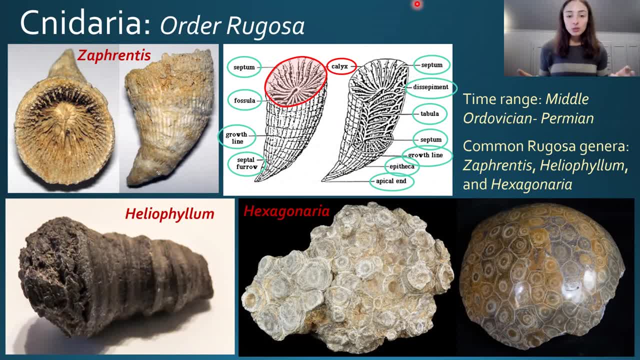 order rugosa. we have here what is nicknamed horn corals, because most of these corals were solitary, So they weren't colonies of different polyps, They were one and they were in these shapes of horns. However, they did have colonial genera, such as the bottom right image where we 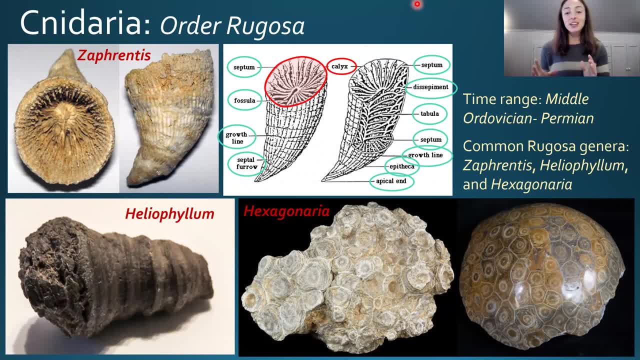 have hexagonaria- I know crazy name, but it's the name of this colonial rugosa coral- But most of them were more like heliophytes, And so these were the three main types of tabulate corals, And so 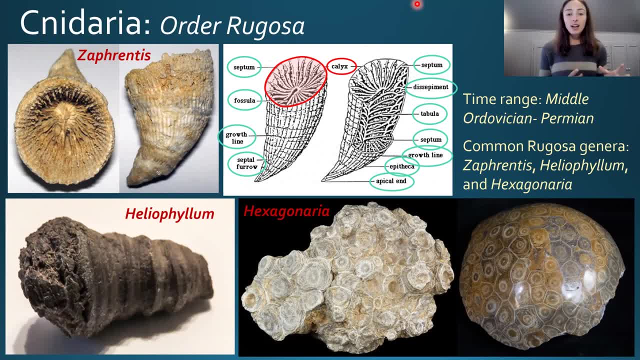 we have phylum and zafrentis in the left side of the slide, And these were solitary, so not colonies, and they were kind of shaped like a horn, However some more pristine horns than others, And so what we see in the more pristine type, zafrentis, is labeled. in the middle of the slide We have a. 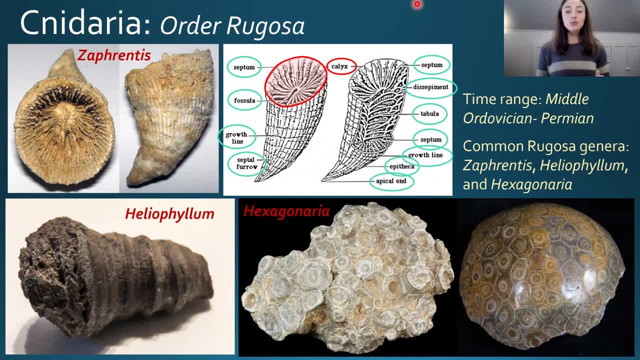 bunch of features on these corals that we're going to go through step by step. So first the calyx, which represents the cup-like portion similar to the corallite on the tabulate coral, but representative of the tabulate coral, And then we have the corallite, which is the corallite on the 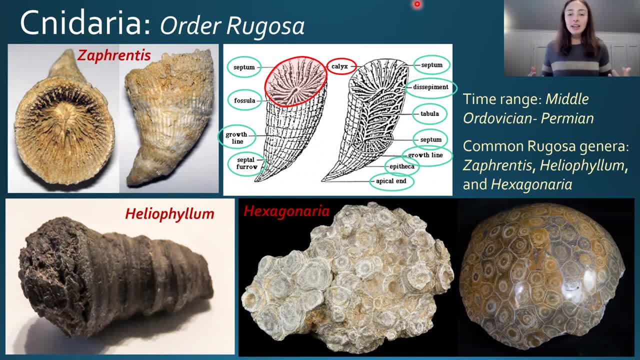 cup-like portion of a solitary horn coral And in the calyx we have the fasula, which represents a big gap in between the forming septa, And all the septa are radial-like separation structures that form throughout the horn coral but are pretty much only seen at the top in the calyx, where we 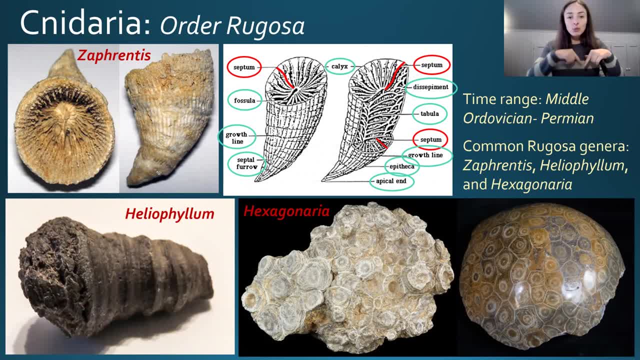 have all of these lines that we can look at, And then the only place we don't have one is in the gap in the fasula, which in Latin fasula is little trench. So now you know why that call it fasula. Then we have septal furrows, which is where the septa affect the outer structure of 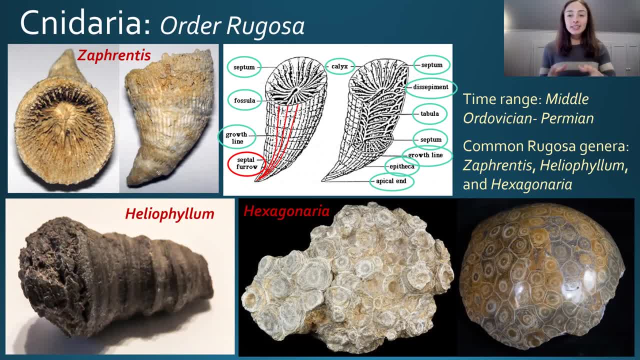 the horn coral and how you can kind of see where the septa are inside of that coral because of the outer structure, furrows. And then you have growth lines which are horizontal on the horn rather than vertical like the septa, And each of these lines represent new growth from the coral as it grows. 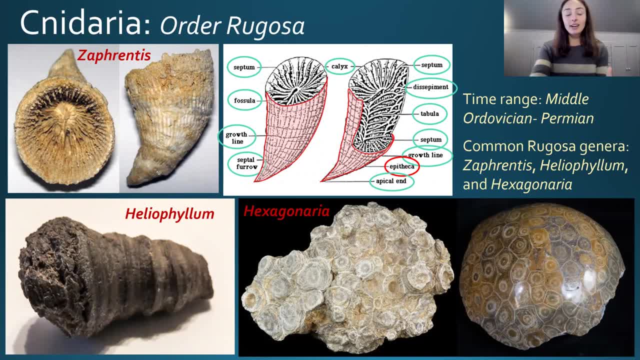 that direction. And then you have the entire body of it, which is called the epitheca, And then you have more internal structure, which is called the epitheca, And then you have more internal structure like tabulae and decepaments, And here they're just pointing out one, So they say tabula and 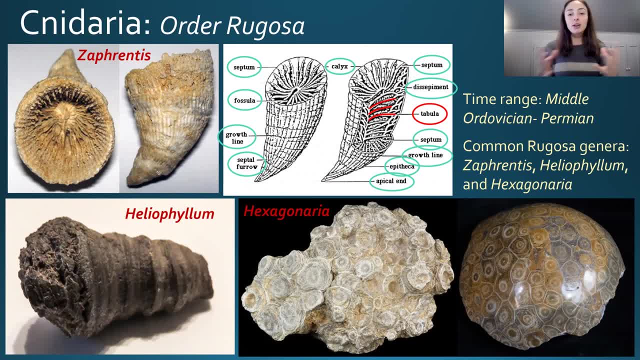 decepament. These are the singular forms of those words. So anyway, the tabulae are highlighted here in the red lines and they're more of the horizontal table-like structures in the internal part of the horn. And then you have the decepaments, which are kind of more bubbly. 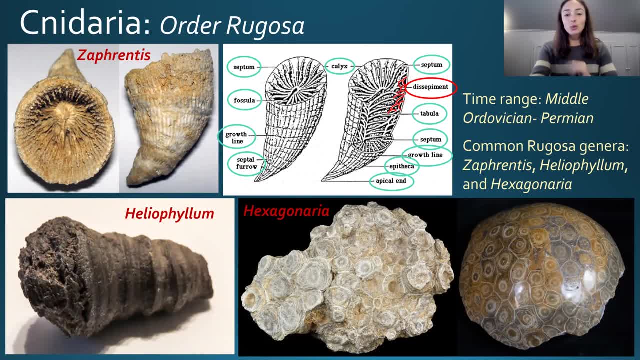 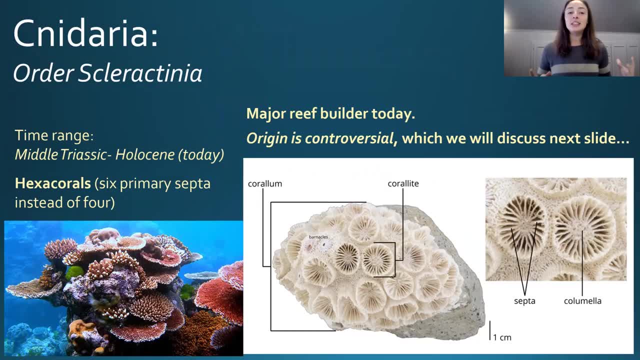 structures on the outer parts, near the edges of the horns, And lastly we have the apical end, which is the point of the horn. Now we're getting into the last order of the subclass Zoantheria within the class Anthozoa, within the phylum Cnidaria. So this order is the 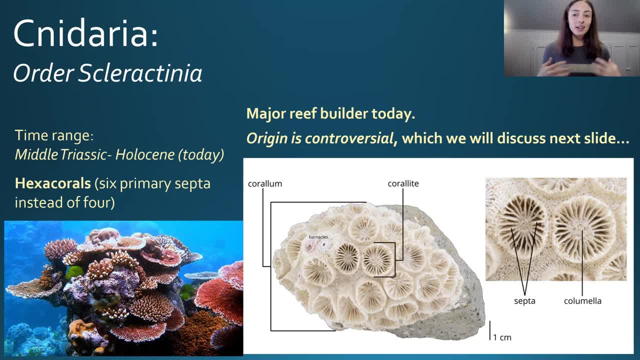 Scleractinian corals. This order, unlike the tabulae and rugose corals, didn't die out in the Permian. In fact, it wasn't even around yet. What happened with the tabulae and rugose corals? 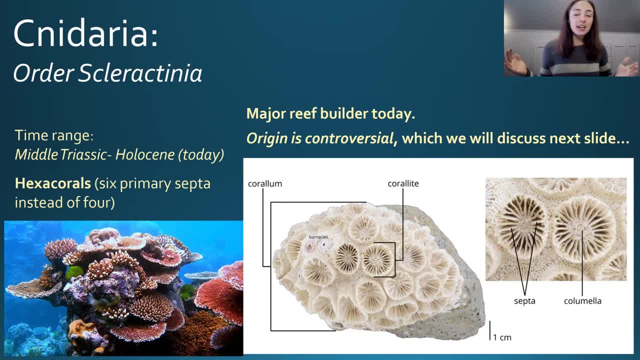 is they evolved way early on in the Ordovician and went extinct at the Permian And unlike that, the Scleractinians actually didn't even come about until the Middle Triassic. So after the Permian all the other corals go extinct. Then you have the Early Triassic, in which there's this hiatus. 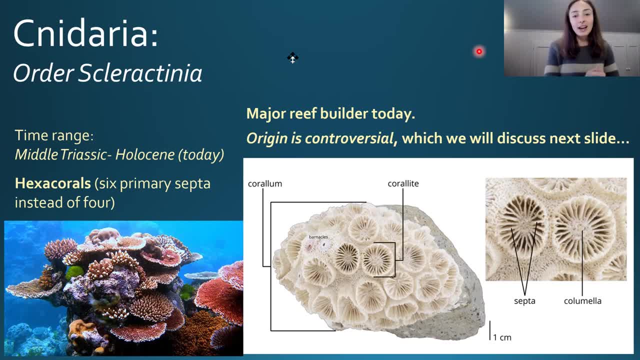 of corals and reforming structures. And then you have the Middle Triassic, where Scleractinia evolved and then start to become reef builders again. This is really interesting because this makes their origin very controversial. What happened in the Early Triassic? Are these? 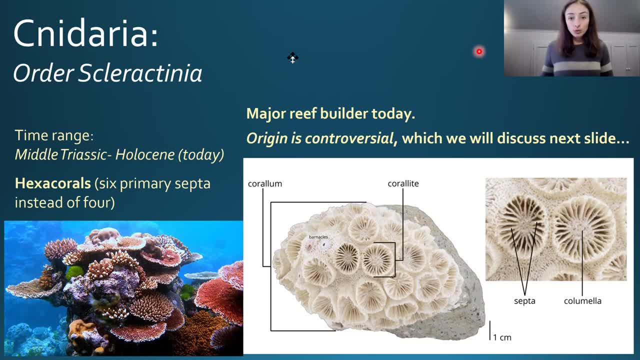 Scleractinian corals, just more evolved groups of rugose corals, or are they a totally different lineage? We don't know, But people think they're separate than rugose and tabulae corals because, even though some of them look similar to rugose corals, they're hexacorals. 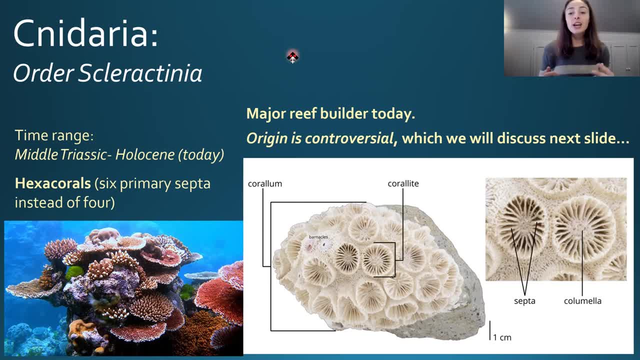 meaning that they have septa that insert 60 degrees from each other and therefore have numbers of septa divisible by six rather than four, like seen in rugose corals. Additionally, we have this time gap, which also makes us think that they're not part of rugose or tabulae. 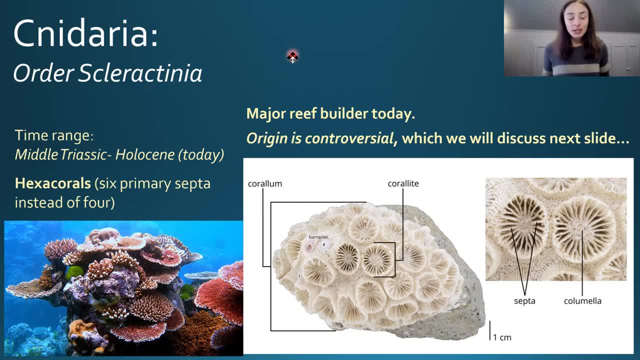 But instead of starting all over again with coral evolution starting from the beginning, which is crazy unlikely- what most likely happened, or what most paleontologists think happened, is that a group of soft-bodied sea anemones that previously weren't preservable. 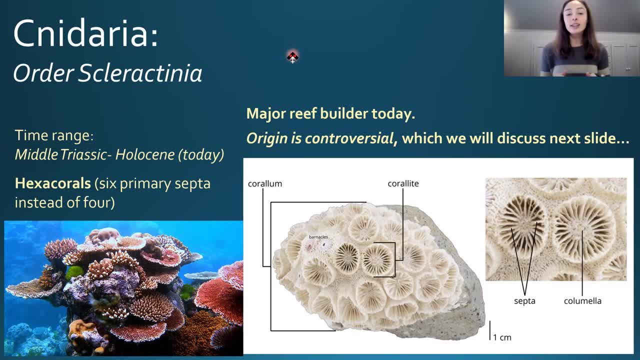 because they didn't have hard parts, evolved the ability to calcify their skeletons and became preservable, which are now represented by the Scleractinian order of corals. And these Scleractinian corals continue today and are the only order of corals left on Earth today. 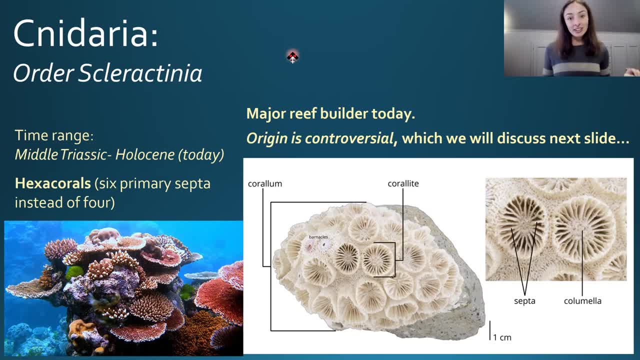 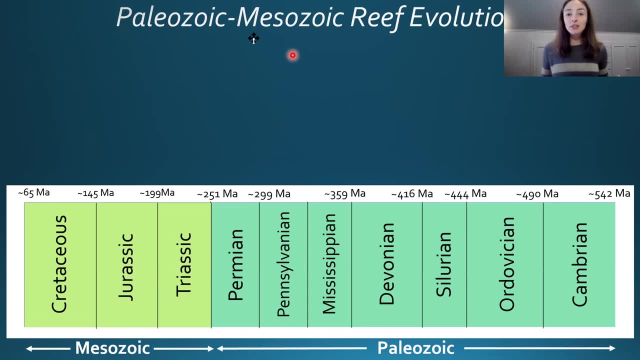 So any live coral you ever see in your lifetime is a Scleractinian. So now I want to discuss evolution. Corals and reef building organisms in general, have gone through a crazy amount of changes throughout the Paleozoic and Mesozoic. So 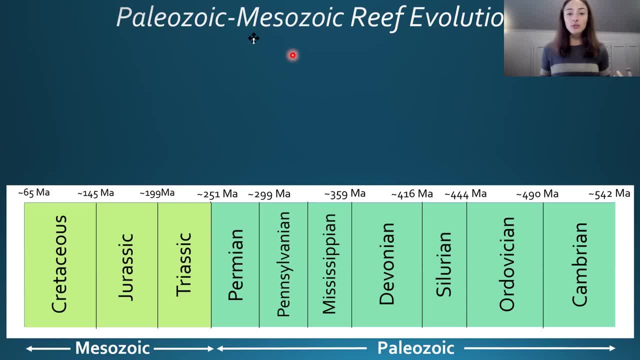 we're going to talk about the different evolutionary events that occurred in all of reef building organisms on this timeline and how reefs evolved as a whole throughout the Paleozoic and Mesozoic. So first we have the Archaeosciathan reefs in the early Cambrian. 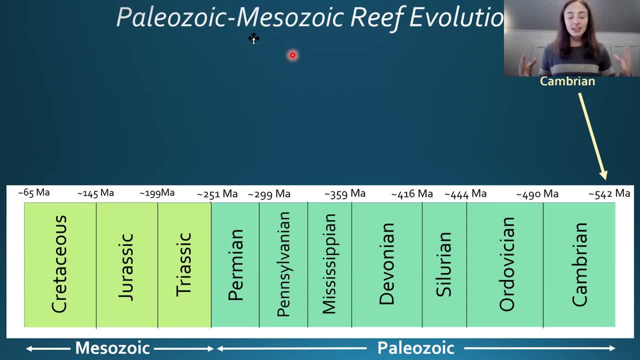 And I'm sorry, I realize that my face right now is probably covering this text. It says Archaeosciathan reefs in early Cambrian. Basically, what we had in the early to middle Cambrian is a reef building group called Archaeosciatha. If you want to know more about the 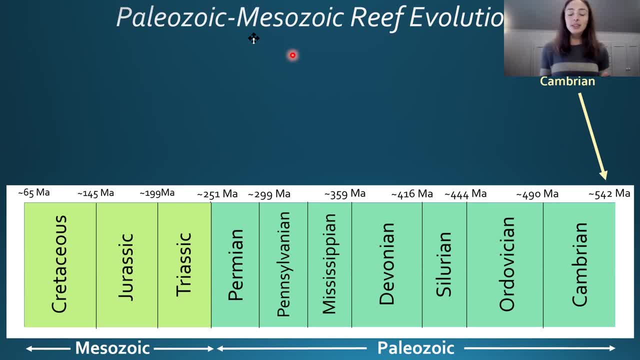 group. you can watch the Periphera video. But basically they only lived until the middle Cambrian- Because they only lived from the early to middle Cambrian and then went extinct. there was a reef hiatus or a gap in reef building organisms or reefs in general. 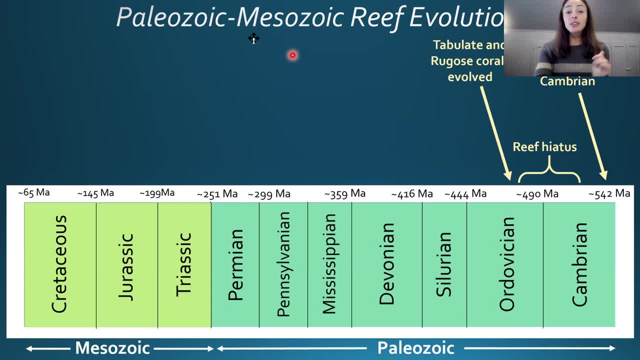 in the middle Cambrian to the early Ordovician, And then you have tabulate corals and rugose corals begin to evolve in the early middle Ordovician, which then allowed reefs to once again proliferate in the Silurian and Devonian, Where we have tabulate and 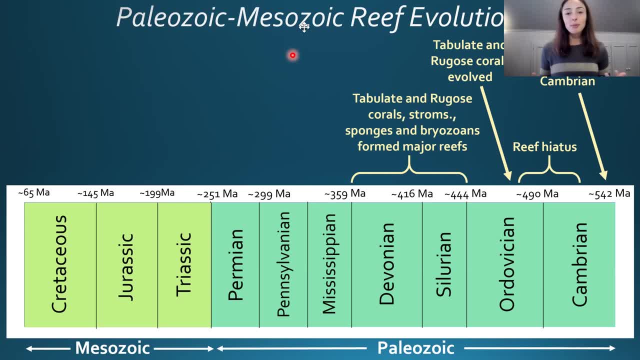 rugose corals, along with stromatoporites and sponges, which we talk about in the Periphera video, along with bryozoans forming the major reefs during these periods. Then we have the Devonian extinction, which really decimated rugose and tabulate corals. After the Devonian extinction. 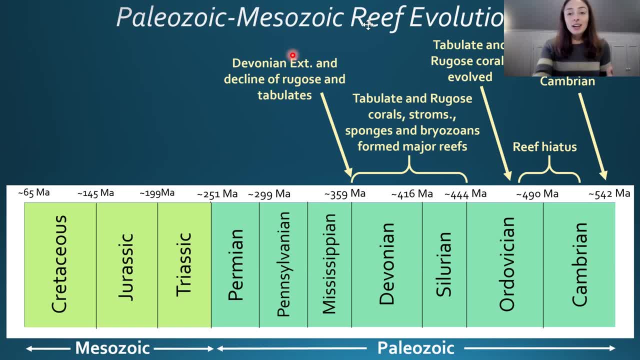 rugose tabulate corals were never as abundant and basically caused another reef hiatus in the Carboniferous or Mississippian and Pennsylvanian periods of the Paleozoic. Because of their decline they weren't able to form major reefs anymore, And then during 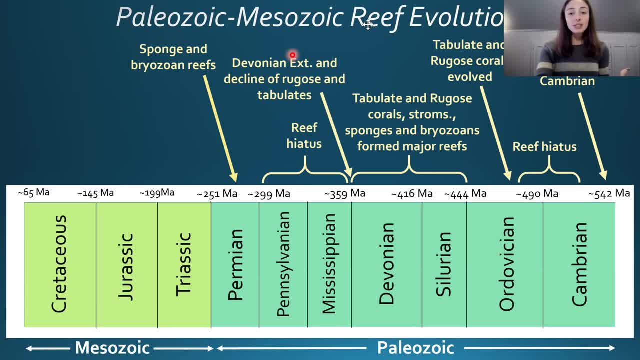 the Permian you had some sponges and bryozoans begin to build reefs again And then the tabulate and rugose corals finally go extinct after straggling on through the late Paleozoic. at the end, Permian extinction. Then you have another reef hiatus because of this extinction. 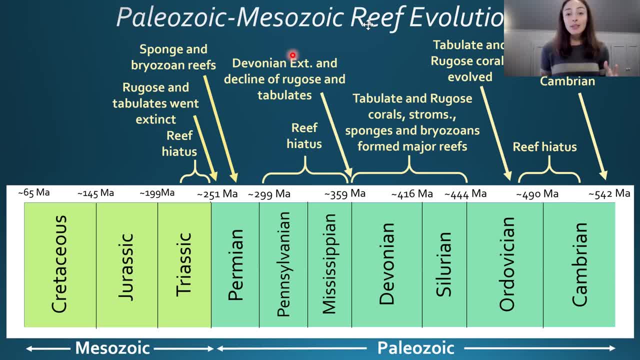 event And from the end of the Permian to the middle Triassic, you have an unknown history of what was going on regarding reefs. Then you have the Sclerotinian corals evolve, like we talked about. unknown origin, probably a calcified sea anemone that hadn't been fossilized and preserved. 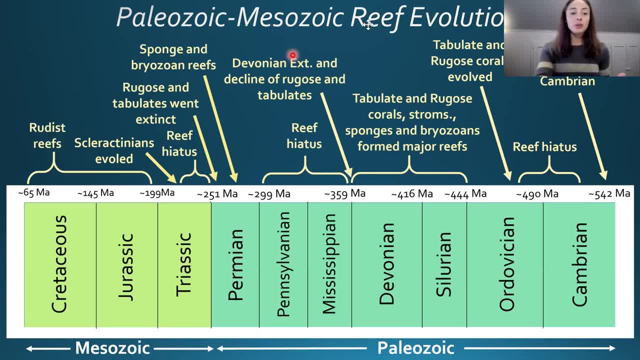 before, so we have no record of it. And so then these evolved and started building reefs again, And then through the rest, of the Mesozoic rudists, which are a type of mollusk we'll talk about in the mollusk video- dominated reef building and reef environments in the Mesozoic. 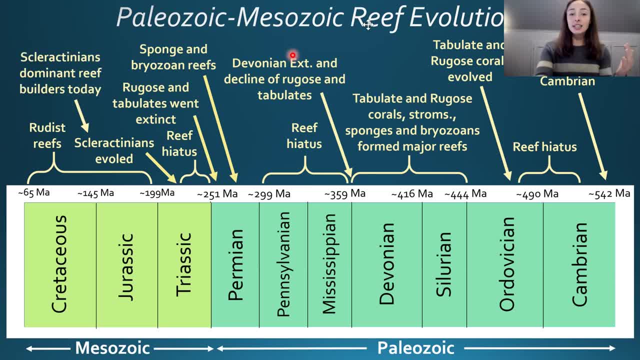 until they went extinct at the end of the Cretaceous, And then Sclerotinians became the dominant reef builders again after the Mesozoic, throughout the Cenozoic, and continue to be the dominant reef builders today. So now for a little bit of Cnidarian ecology. this is going to be: 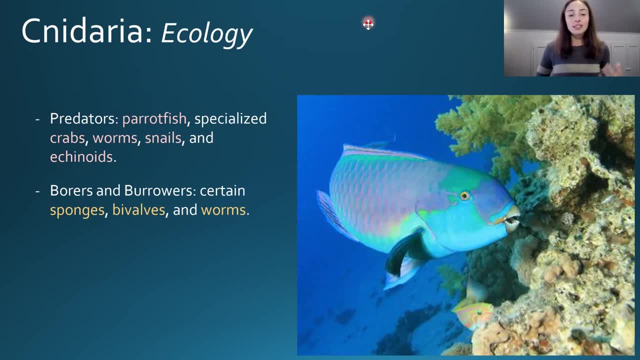 pretty short. Basically we're going to be talking about the Cnidarian ecology of the Mesozoic. Basically, we know that predators of corals include things like parrotfish- shown here in the right- and certain crabs, worms, snails and echinoids, But basically they're pretty safe. 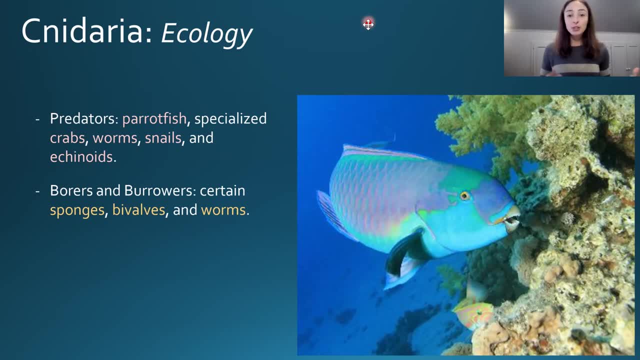 I mean they have mutually beneficial relationships, more so than they have predator-prey relationships, except when it comes to humans, And we'll talk about how we can be killing corals more than any other predator in the sea a little bit later, in a different slide. However, 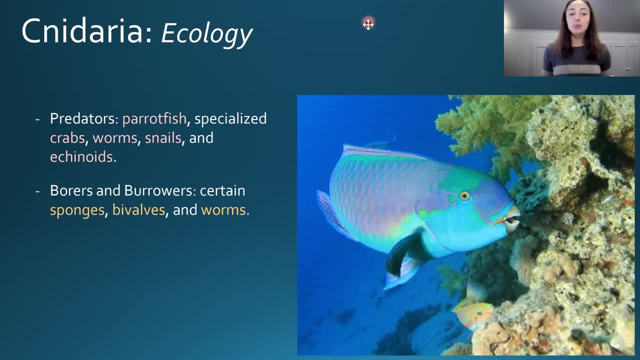 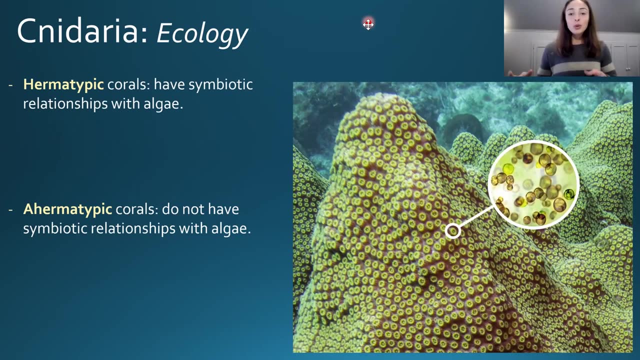 before we get to that, we must mention that there are also animals out there that burrow and bore into corals, such as sponges, bivalves and worms, And then we'll have different types of corals that can live either with a symbiotic relationship with algae. 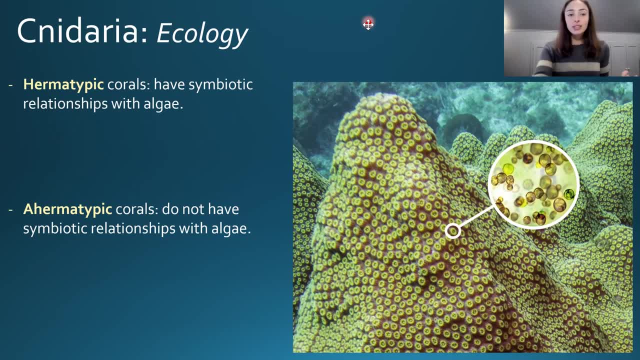 or without that relationship. And so when corals do live in a symbiotic relationship with algae and contain algae called zooxanthellae inside their polyps to grow, they are called hermatypic corals. The algae is called zooxanthellae and these corals are restricted to clear 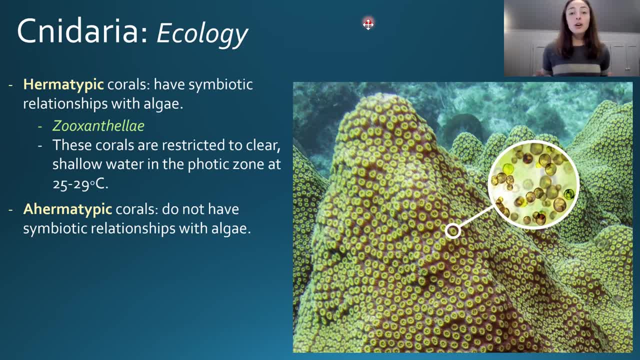 shallow water in the photic zone because the algae needs sunlight to photosynthesize And their temperature range is very strict compared to the ahermatypic corals, which can live in deeper, colder waters, down to one degree celsius, And they don't need sunlight to grow. However, 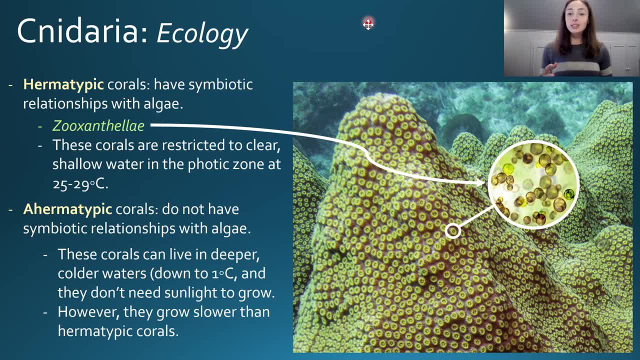 they do grow slower than the hermatypic corals and therefore it is thought that these algae somehow give the hermatypic corals energy boosts or food boosts or some sort of boost to grow faster. But not everything is known about it. so if you'd like to look into it and study these things, 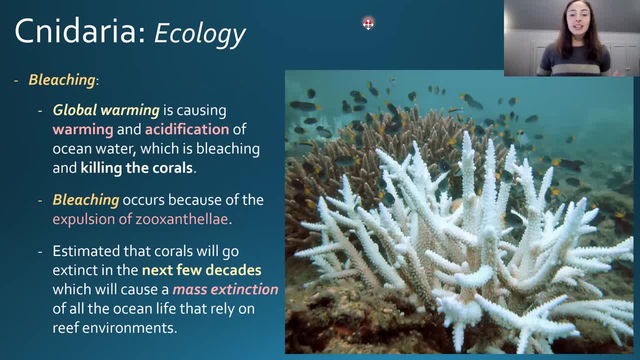 they're really amazing. You should go for it. The last thing that I want to discuss is bleaching, because how can we talk about corals without talking about this? We talked already about how there are pretty few predators for corals. However, they have a lot of potential for. 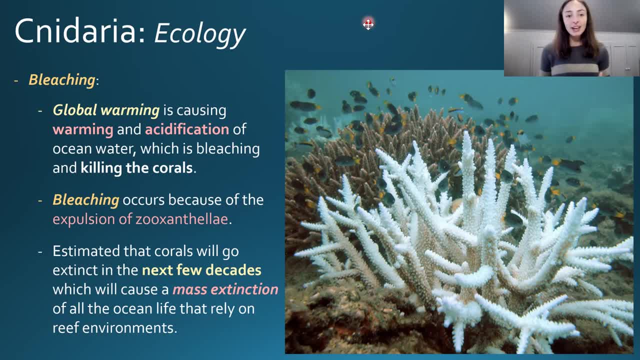 their health. They are dying at unfortunate rates because of global warming. Global warming is causing the warming and acidification of the ocean, two major factors in killing corals, which host major ecosystems and marine environments. Acidification will literally just dissolve corals, But bleaching is what occurs when the warming of the ocean water 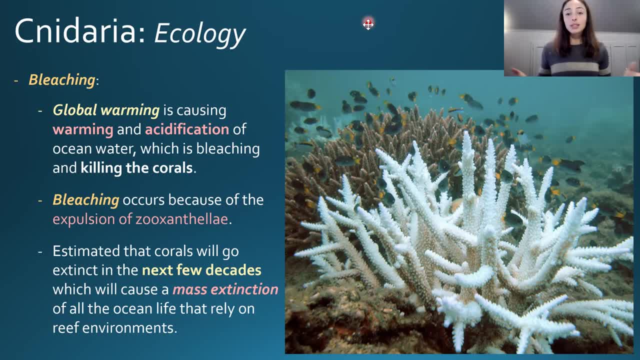 causes the algae in symbiotic corals to expel out of the polyps and just leave the coral, even though it relies on this algae. So when this zooxanthellae algae gets expelled, the coral is left bleached and without the algae to come back, it will eventually die. 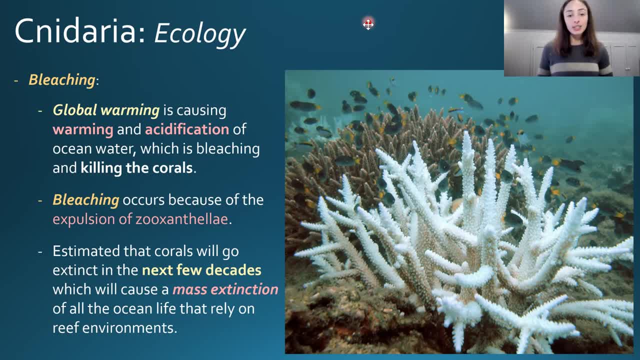 It is, unfortunately, estimated that all corals will go extinct in the next few decades, and so this will cause huge mass extinctions of all of the ocean life that relies on reef environments, And so it's important that we understand this, just to understand how.